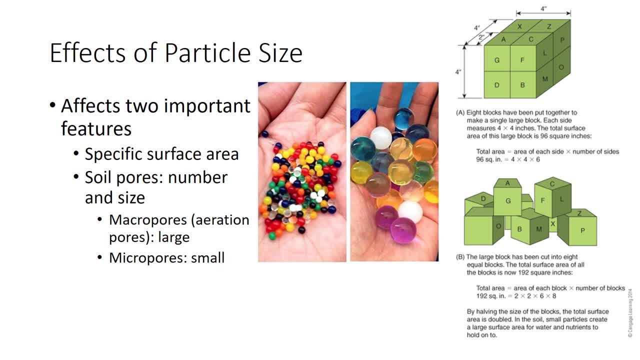 Droplets clinging to the surface of the marbles are the only water retained in the pile, because water cannot soak into the marbles Following the rule about particle size. a pile of small beads holds more water than a pile of marbles because it has more surface area for water. 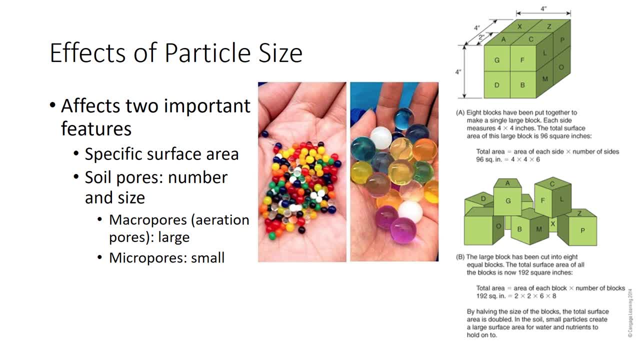 to cling to. Because soils with the smallest particles, like silt and clay, have the largest surface area, they hold the most moisture. Reactions that hold plant nutrients in the soil also occur on particle surfaces. Therefore we can make the rule that the smaller the particles 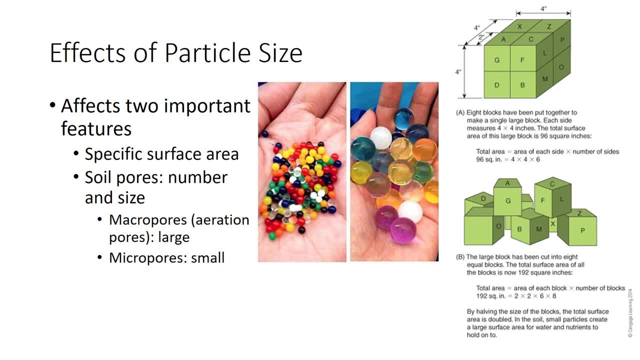 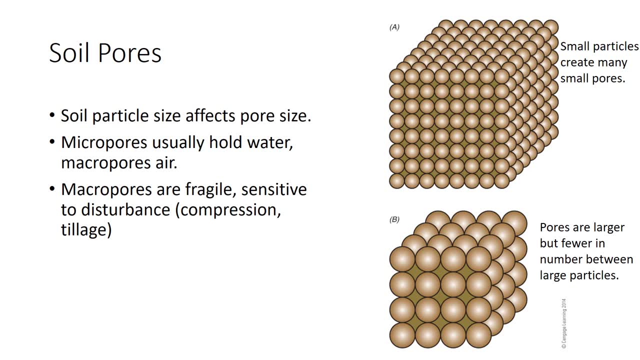 the larger particles stored in soil are, the more water and nutrients the soil can retain. Pore size and number also depend on particle size. The figure suggests that more pores are found between small particles than between large ones. The figure also shows that pores 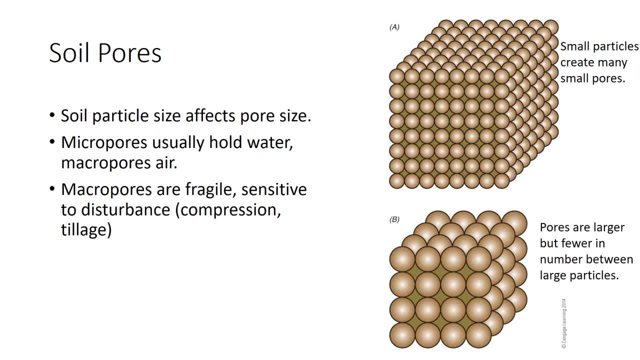 are larger between larger particles. The soils high in clay have many small pores, while soils high in sand have fewer but larger pores. The larger pores, called macro-pores or aeration pores, create the easiest pathways and so largely determine the movement of air and water through. 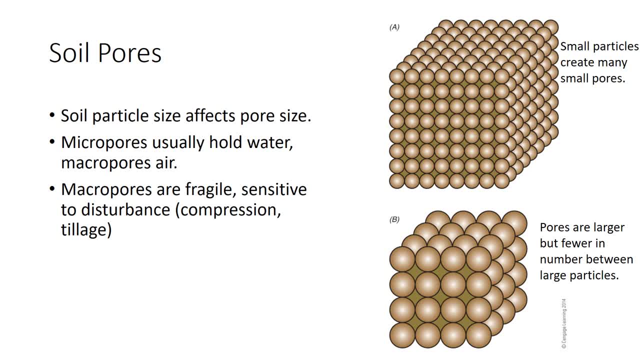 the soil. As water drains down through the soil, it pulls air in behind it which occupies the macropores. Small pores or micropores retain some water as it drains down through the soil. In such small pores, water films surrounding adjacent particles merge holding. 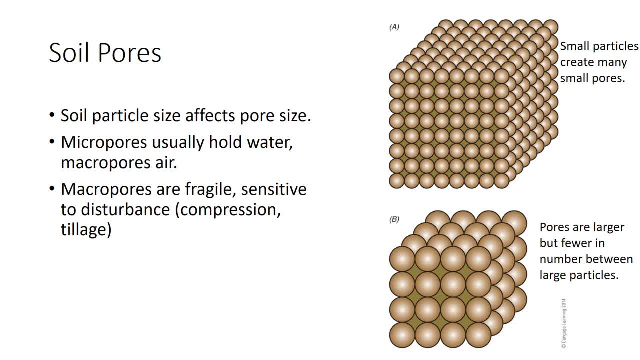 water in place, but excluding oxygen. Further, because of the small pore size, micropores make difficult pathways for water movement. Sometimes the larger micropores distinguish as mesopores medium-sized pores that hold readily plant-available water. It is worth. 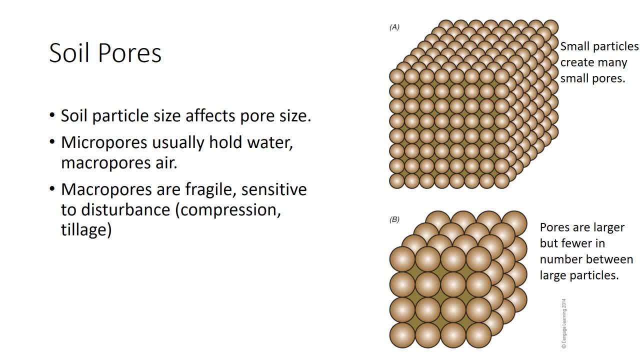 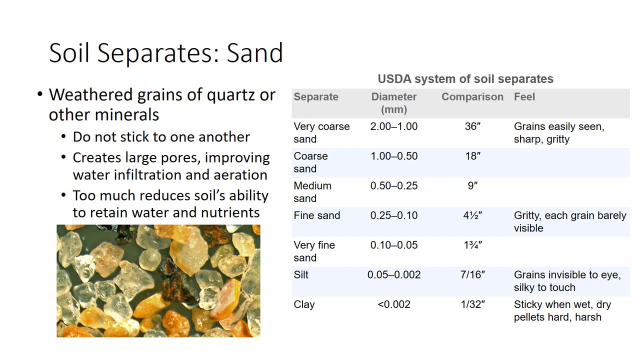 noting that macropores are fragile, sensitive to disturbance. These pores tend to collapse when compressed or exposed to tillage, even or especially by rototillers Reducing Macroporosity. Soil scientists divide mineral particles into size groups called soil separates and define. 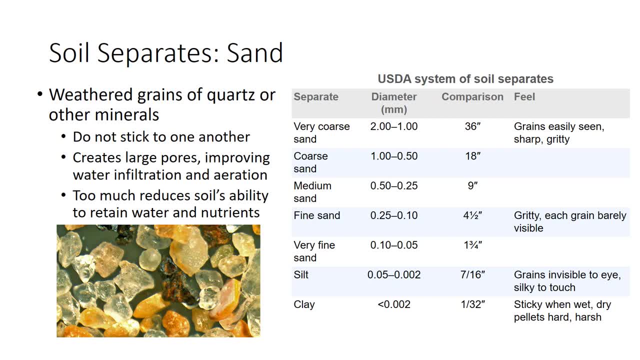 three broad classes: sand, silt and clay. These three together make up the fine earth fraction of soil used to determine texture. Larger particles, such as gravel, are considered to be coarse fragments and are not considered in texture. The table names the separates. 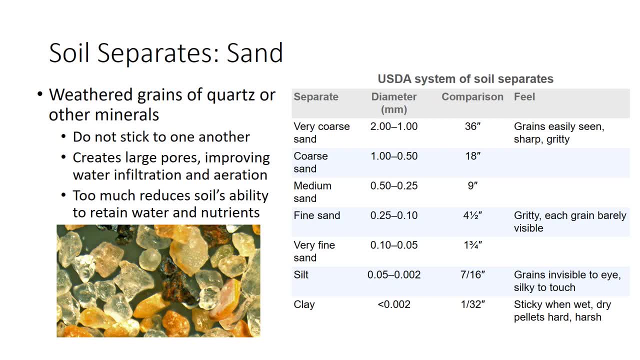 and gives their sizes according to the system adopted by the United States Department of Energy. The comparison shows the difference by setting a very coarse sand grain equal to three feet in diameter. Sand, the largest soil separate, is composed mainly of weathered grains of. 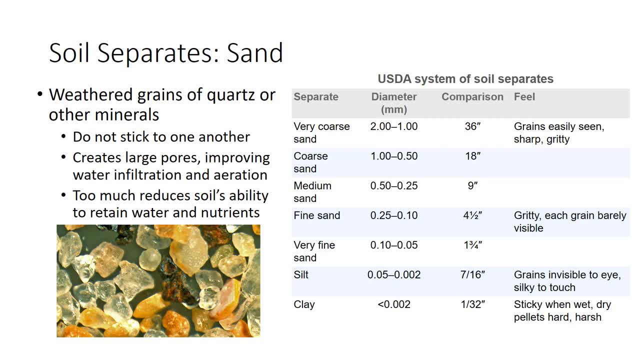 quartz and other minerals. Sand particles are further divided into five subcategories, as shown in the table. Individual sand grains, except for very fine ones, are visible to the naked eye. All are gritty to the touch. Sand grains do not stick to one another, so 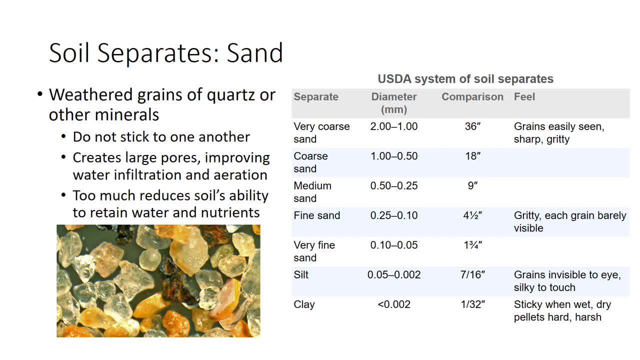 they act as individual grains in the soil. Enough sand in a soil creates large pores, so sand improves water infiltration and aeration. On the other hand, large amounts of sand lower the ability of the soil to retain water and nutrients. Silt is the medium-sized soil. separate Silt particles are silky or powdery to the touch. 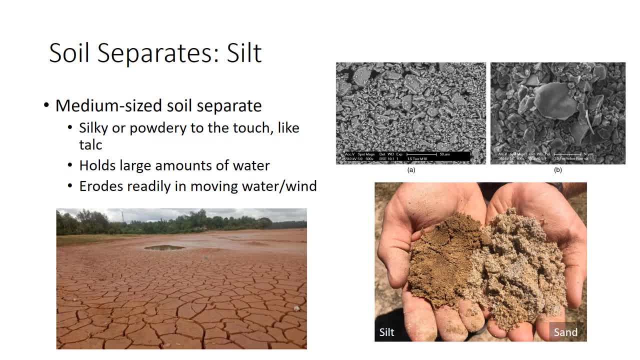 like talc, Like sand, silt grains do not stick to one another. Soil separators are smaller and upscale. They will be separated in two glory forms. where two grains are separate, soil separates. silt has the best ability to hold large amounts of water in a form. plants. 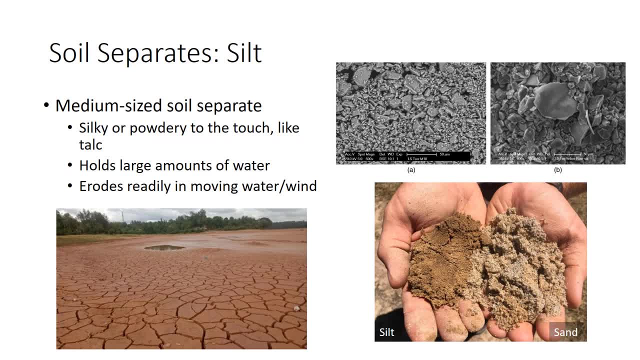 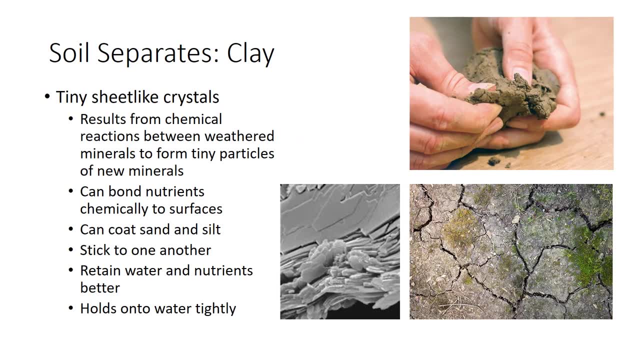 can use. Silt, however, erodes readily in moving water and wind because of its size and lack of stickiness, which holds clay particles in place. Clay is the smallest soil separate, consisting mostly of tiny sheet-like crystals. Clay particles are about the size of particles in tobacco smoke, While sand and silt result simply from. 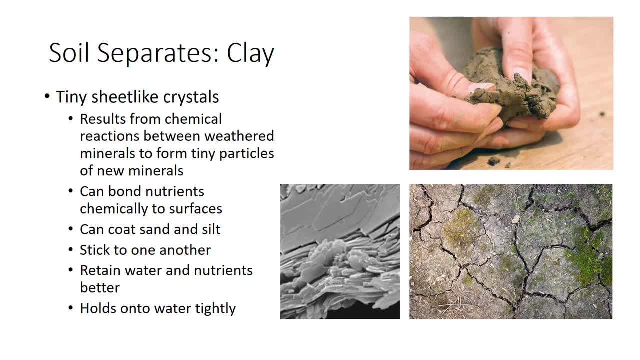 rock crumbling into small particles. clay results from chemical reactions between weathered minerals to form tiny particles of the new minerals. These new minerals are able to bond nutrients chemically to their surfaces, holding plant nutrients in the soil. Particles the size of clay, unlike larger ones such as silt or sand, can move through the soil filtering. 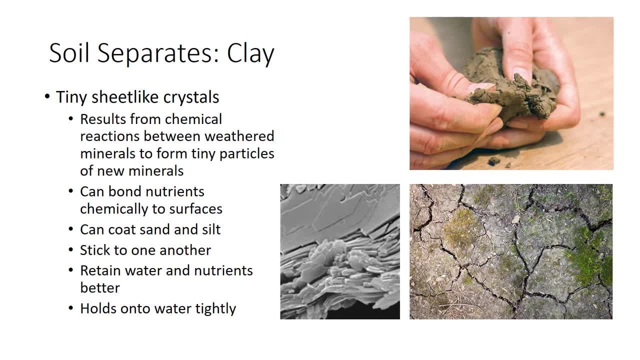 between larger particles in moving water. This is a natural process of soil formation. An example of translocation and alluviation is the formation of soil particles in the soil, which often leads to subsoils enriched in clay. Also, as a result, clay often appears. 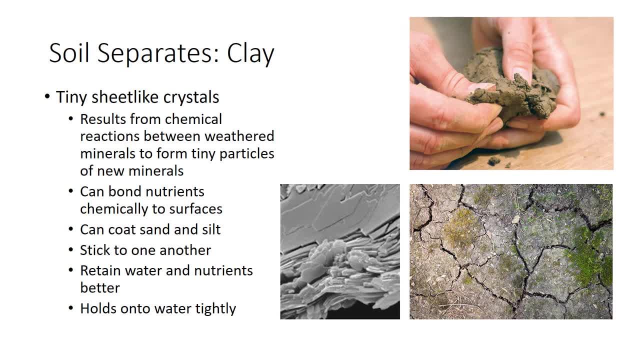 as coatings on sand, silt or larger soil units. Clay particles stick to one another and so do not behave as individual grains in soil. This helps prevent them from being carried away by wind and water. Wet clay is usually sticky and can be molded Some types. 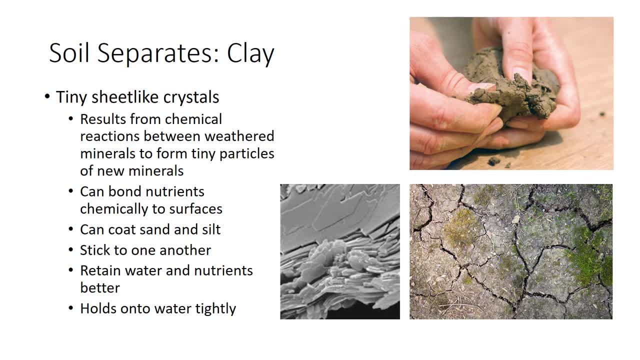 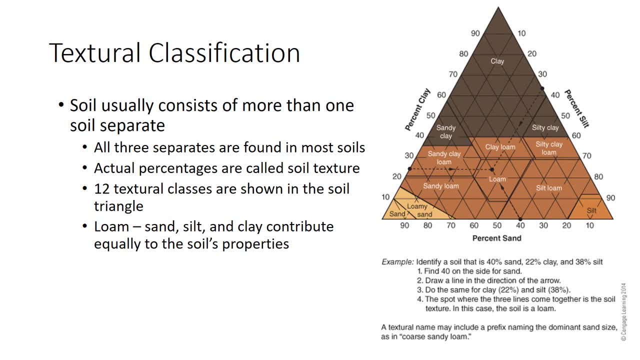 of clay swell when wet and shrink as they dry. Soils usually consist of more than one soil separate. All three are found in most soils. The exact proportion or percentage of all three separates is called soil texture. Obviously, any number of combinations of the three is possible. 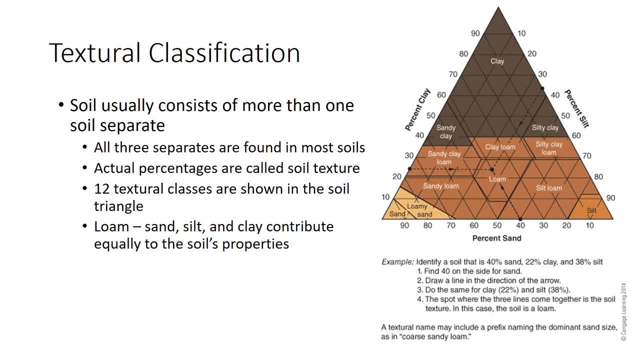 so soil scientists simplified texture by dividing soils into textural classes. Soils in the same textural class are similar. The 12 textural classes are shown in the soil triangle in the figure. Each side of the triangle represents the percentage of one soil separate A person. 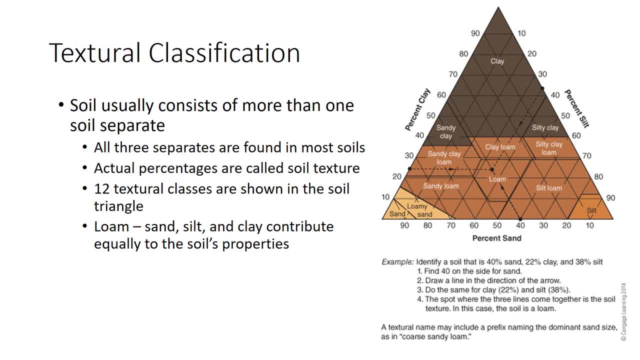 can measure the amount of soil in each soil separate. A person can measure the amount of sand, silt and clay in a soil sample and simply read the class from the triangle. For example, if you have 40 percent sand, 38 percent silt and 22 percent clay, the 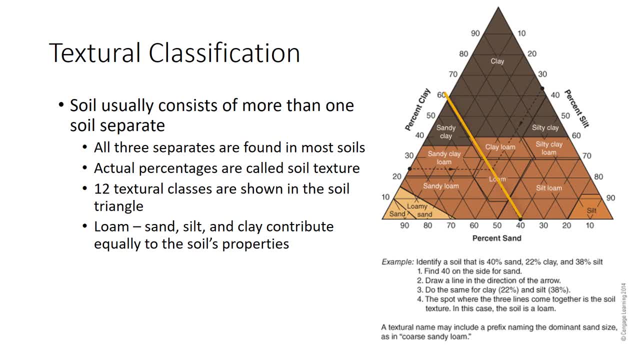 first step is to find 40 percent on the sand axis And then draw a line parallel to the silt axis. The next step is to find either 38 percent silt or 22 percent clay. If you choose clay, look for 22 percent on the clay axis and draw a line parallel to the sand. 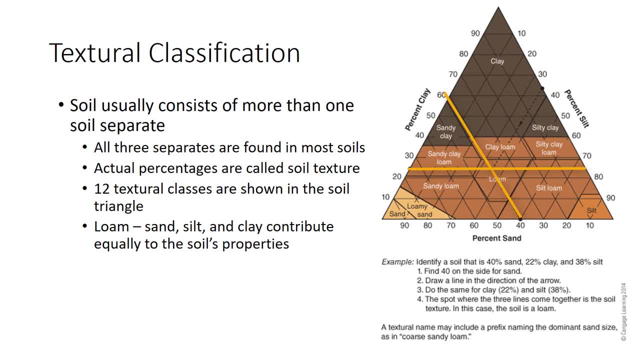 axis to intersect the previous line. If you choose sand, look for 22 percent on the clay from the sand axis. The part of the triangle where the two lines intersect indicates the class of the soil texture. In this case it would be classified as a loam. A loam is a 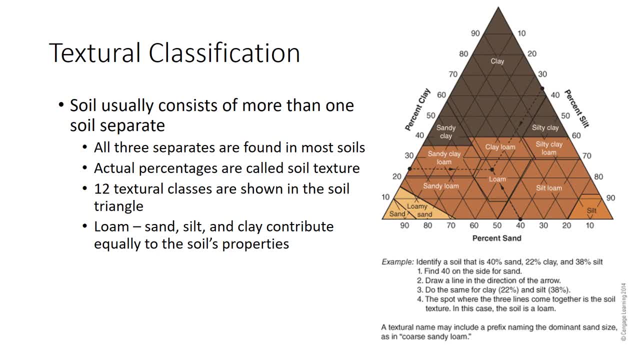 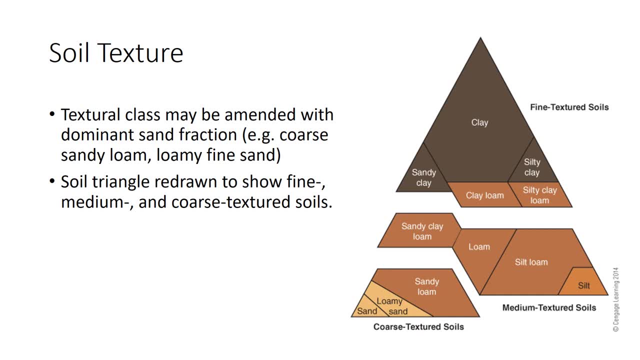 soil in which sand, silt and clay contribute equally to the soil properties. Sand particle size greatly influences soil properties. So for the sandier soil textures the textural class name may be amended by noting the dominant sand fraction One might. 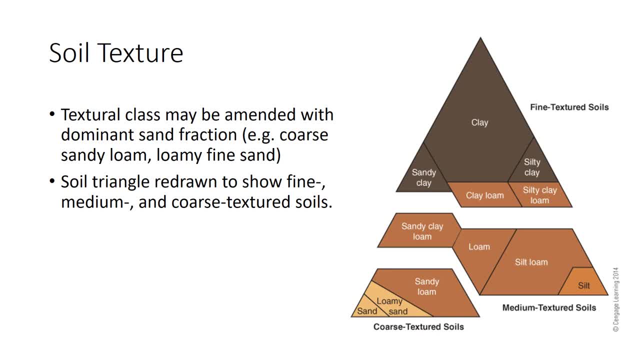 have not just a sandy loam, but a coarse sandy loam, Not just a loamy sand, but a loamy fine sand. Also, in soils high in coarse fragments, the fragment name may be used as a modifier, as in gravelly loamy sand. Growers can usually manage soils without knowing the exact soil. 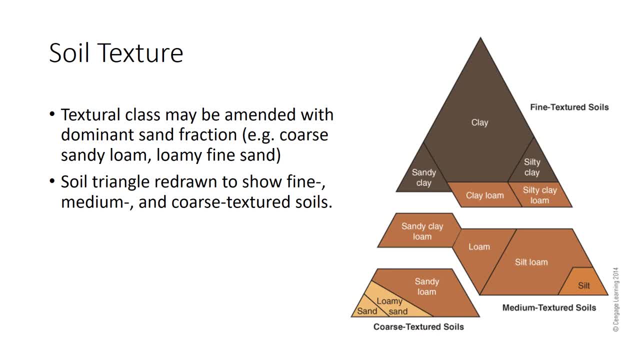 texture, so a broader classification is often adequate. One can simply classify soils as sandy loamy or clayey, as described previously. The figure shows another approach. The 12 classes are divided into three broad categories: coarse, medium or fine. based 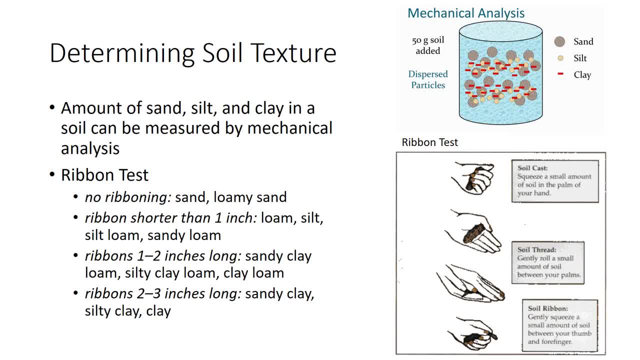 on size of the soil separates. The amount of sand, silt and clay in a soil can be measured by mechanical analysis. Mechanical analysis is based on the fact that the larger a soil particle, the faster it sinks in water. In mechanical analysis one stirs soil into water and notes how fast soil particles settle. 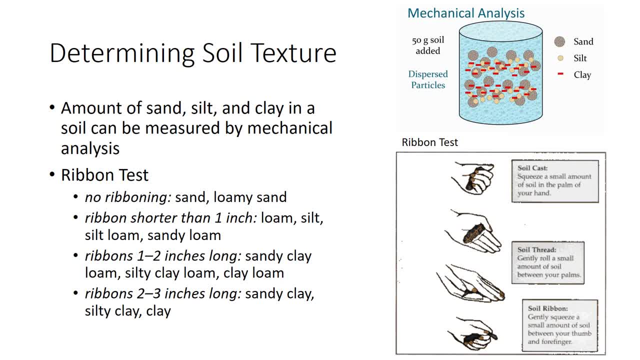 out. This can be observed by performing a sedimentation test. In this test, one measures the depth of sediment at various time intervals to determine percentage of sand, silt and clay, or by using a hydrometer to measure water density at various time intervals. 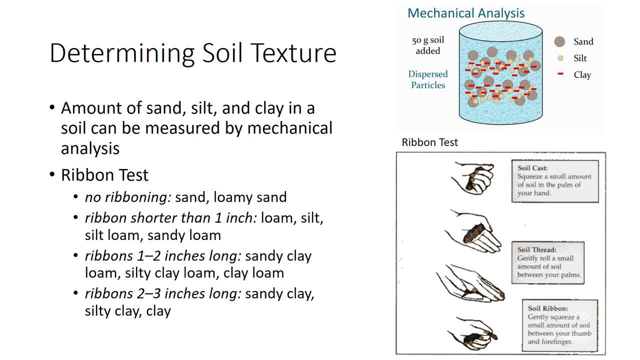 An even simpler test which can be performed on-site is the ribbon, or field test. The test is based on the feel of damp soil and how easily it can molded. All who work with soil, including horticulturists and landscape designers, should be able to perform ribbon. testing. It is based on how long a ribbon will last for wood to become gone, or up to 10 days. It can also be done at a tree or lashing and嗎ackoliatt 놓 trying to make the%. Byこんな way one may also measure the innecessary 난ib and saw resistance just in. 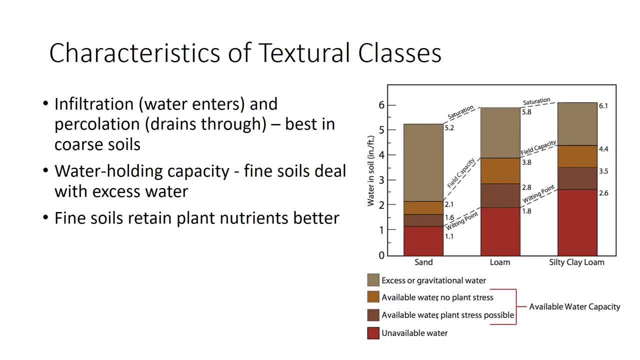 be formed from the sand before breaking Soil. scientists place soils in textural classes because each class has properties important to its management. One can only generalize about textural effects, because other properties also affect the soil. However, here are a few useful guidelines. 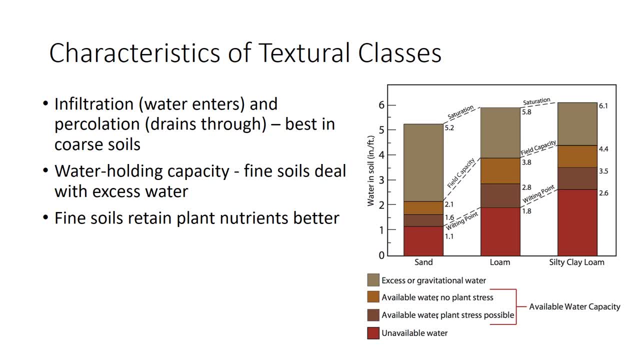 Texture governs the way water behaves in the soil. For instance, water enters and drains through coarse soil most rapidly because of the large pore spaces. Thus a coarse soil dries out most quickly after a heavy rain or in the spring, allowing a grower to get into the field more quickly. 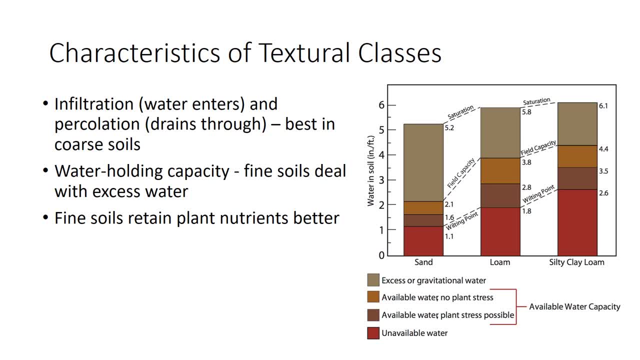 Similarly, coarse soils are more likely to need frequent irrigation. Growers with fine soils are likely to worry about the opposite problem: dealing with excess water. Fine soils retain plant nutrients better than coarse soils. This is true partly because the rapid percolation of water through coarse soil leaches out nutrients. 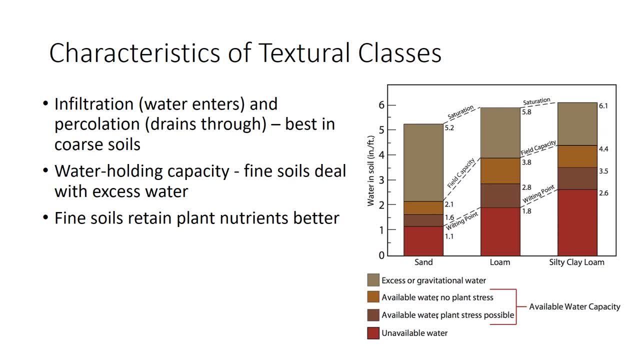 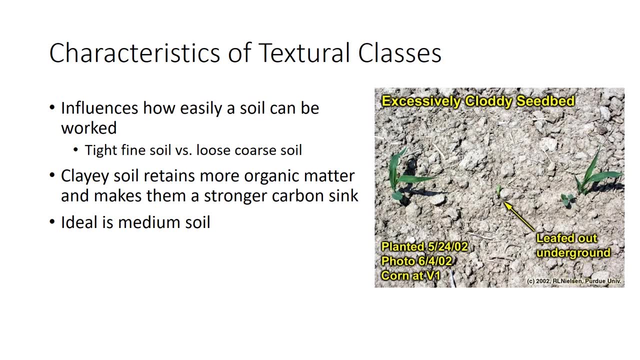 Also, clay particles have the best ability to retain nutrient chemicals. Soil texture influences how easily a soil can be worked. Because clay particles stick together, it takes more horsepower and fuel to pull tools such as plows through a fine soil. Landscapers also find it harder and slower to dig holes in fine soils for planting trees. 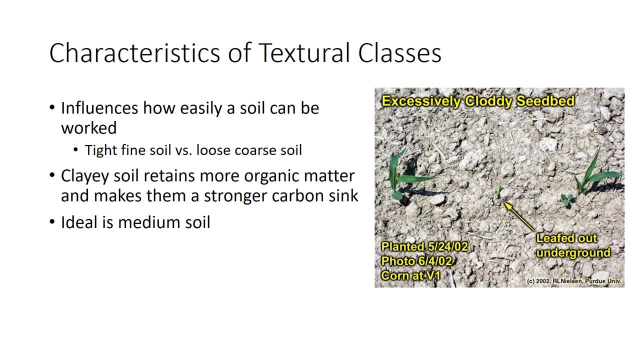 so texture can even affect what should be charged for landscaping services. In fact, soil texture strongly affects many landscape practices. Soil texture can even affect what should be charged for landscaping services. In fact, soil texture strongly affects many landscape practices. Soil texture can even affect what should be charged for landscaping services. 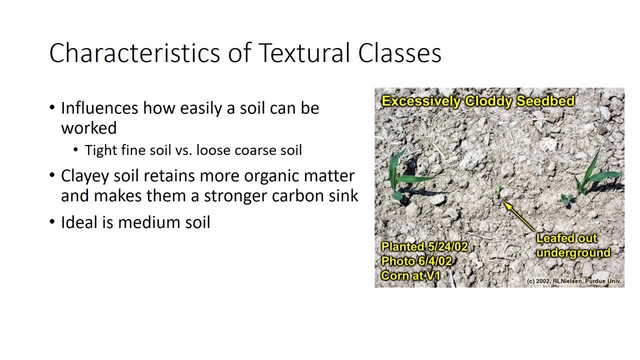 Such as how to design a landscape irrigation system or a retaining wall. The stickiness of clay also affects the condition of the soil. For instance, fine soils often form clods when they are tilled. A crust may also form on the surface and interfere with seedling emergence. 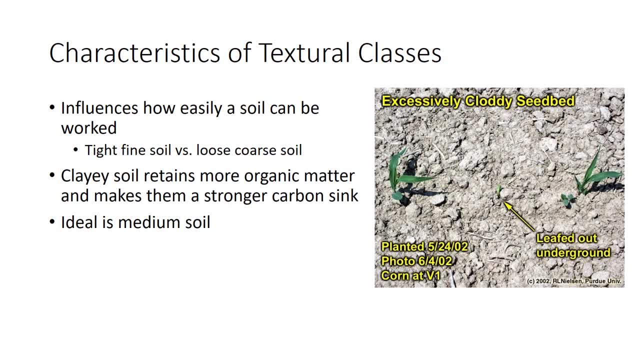 A fine soil tends to be tight, meaning it has mostly small pores that are difficult for air and roots to penetrate. In contrast, coarse soils are loose and well aerated. These soils tend to retain more soil- organic matter than sandy soils, which lends them. 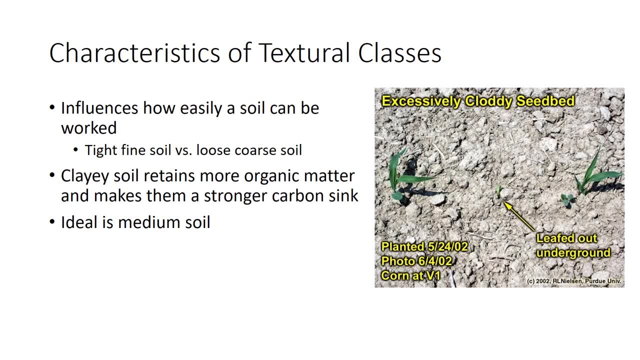 a darker color. The higher organic matter content also makes them a stronger carbon sink, so efforts to sequester carbon will be most effective in finer texture soils. For most purposes, growers consider medium soils to be ideal. They hold water but they do not stay wet too long. 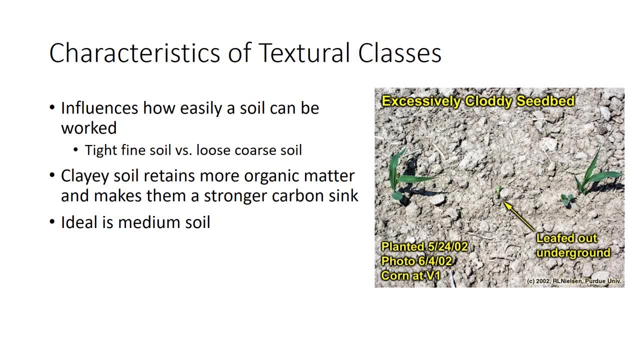 They are neither sticky nor hard to work. In general, medium soils have good traits of both coarse and fine soils, but they are not as good as coarse and fine soils. In general, medium soils have good traits of both coarse and fine soils, but they are 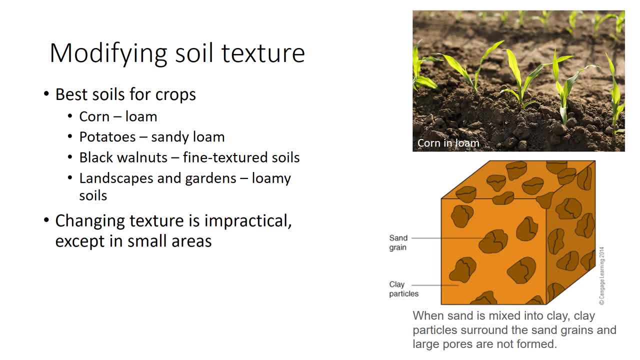 not as good as coarse and fine soils, without their bad traits. Growers and engineers use soils for many purposes. For each purpose, a different soil texture may be best. For example, corn tends to be most productive on a loam, potatoes on a sandy loam and black 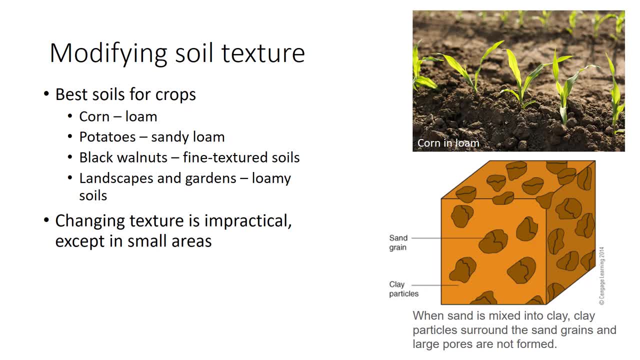 walnuts on fine textured soils. Loamy soils are easiest to use for landscapes and gardens. Can a grower change soil texture to improve it for the crop being grown? Except in very small areas such as golf greens or potting soils, changing texture is impractical. 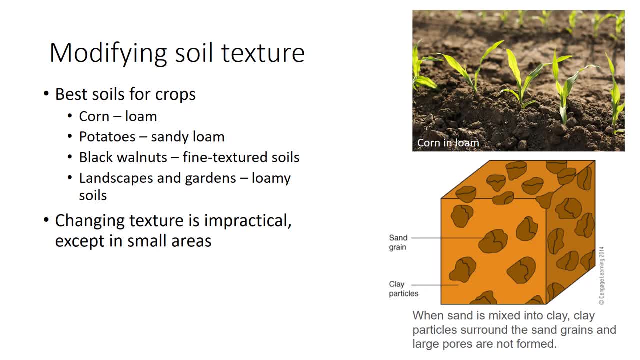 If a grower changes soil texture to improve it for the crop being grown. except in very small areas such as golf greens or potting soils, changing texture is impractical. The amounts of clay or sand to be added are too large. The figure shows the effect of adding sand to a clay soil to loosen it. 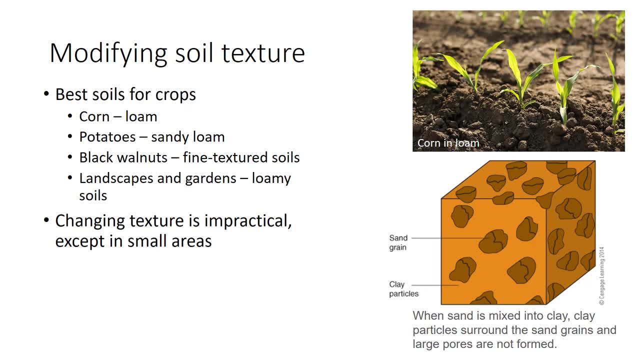 Clay particles surround the sand grains and fill in any pores that may be created. As a result, the soil continues to behave much like clay. To greatly modify clay, enough sand must be added to make the sand grains touch each other and form bridges that exclude clay from the pores between the sand grains. 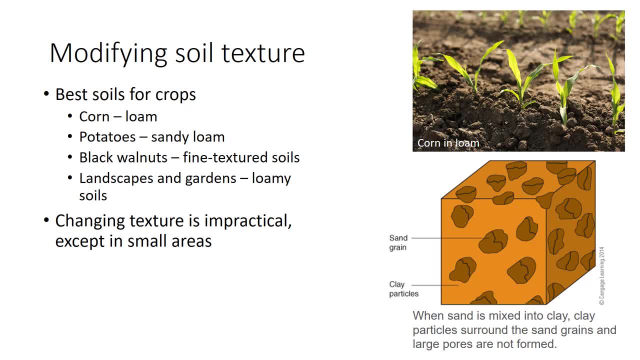 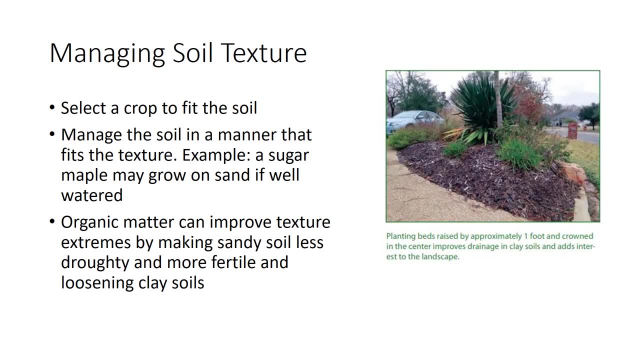 A better way to improve clay soils is to add or add organic matter, a practice described repeatedly elsewhere in this video series. There are three ways for growers to take texture into account. First, select a crop to fit the soil or purchase land that suits the crop. 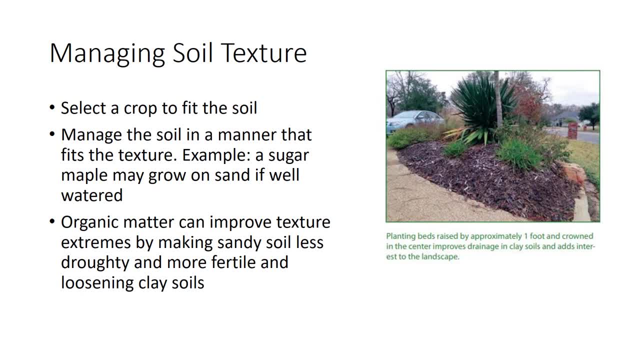 For example, an apple grower may purchase land with a fine soil on which apples grow best. In many landscapes, a sugar maple will not thrive on a sandy soil, while a red maple might do well In other landscapes, a sugar maple will not thrive on a sandy soil, while a red maple 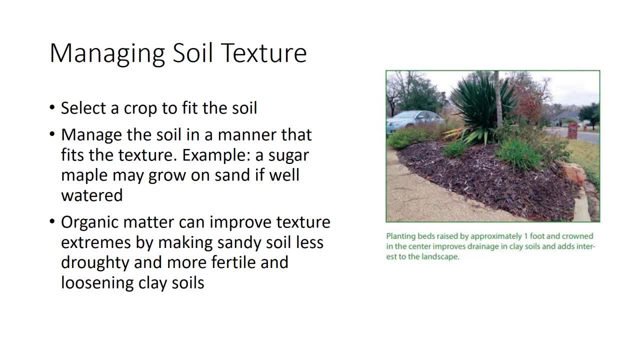 might do well. An axiom of landscape design is: put the right plant in the right place, And texture is an element of that. Second, manage the soil in a manner that fits the texture. For example, with proper fertilization and irrigation, coarse soils can be very productive. 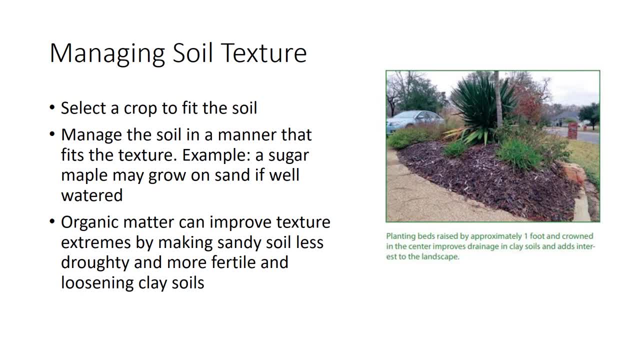 A sugar maple may grow on sand if well watered. When planting landscape trees in Minnesota many landscapers plant high and heavy clay soils. That is, the top of the root ball will be a couple of inches above grade with a bit of soil added around it. 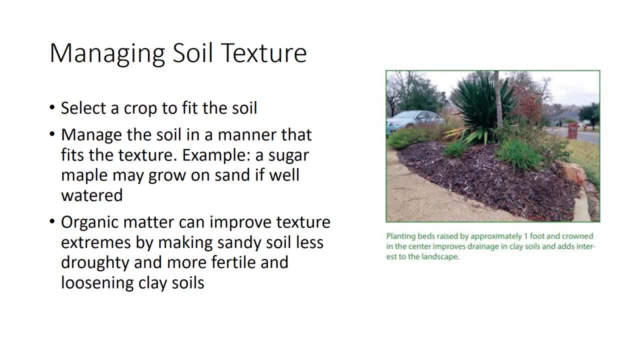 This is a good example of how to manage soil in a manner that fits the texture. Third, organic matter can improve texture extremes by making sandy soils less droughty and more fertile and by loosening clay soils. The third choice might be considered one of the cardinal rules of soil management. 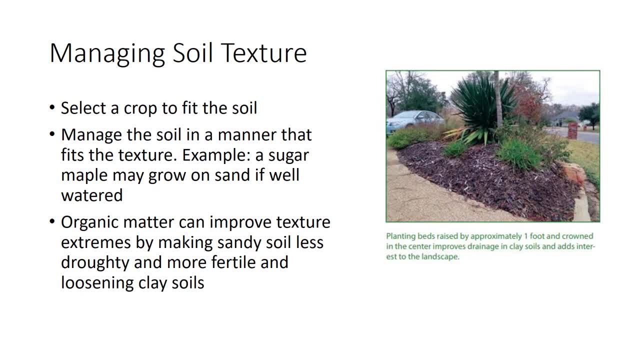 Add organic matter to improve soil. It might be pointed out that adding organic matter does not actually change soil texture itself. Think about the definition of soil texture to determine why. It does, however, modify another powerful physical property, to be discussed in another. 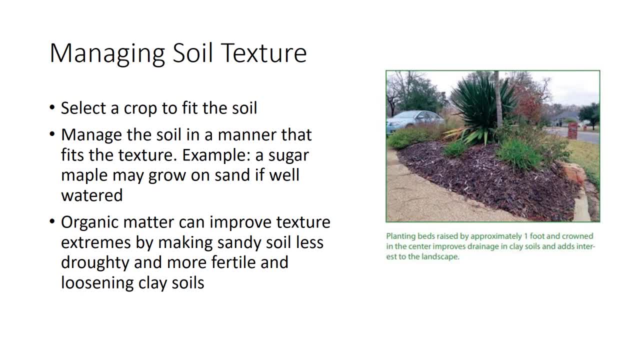 video soil structure. In conclusion, the most basic physical property of soil is texture. the proportion of sand, silt and clay Texture strongly affects how growers use soil.